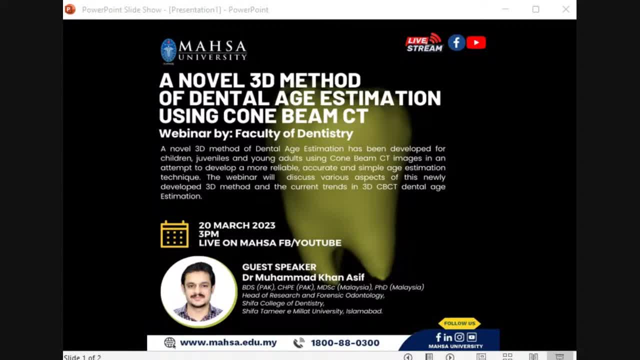 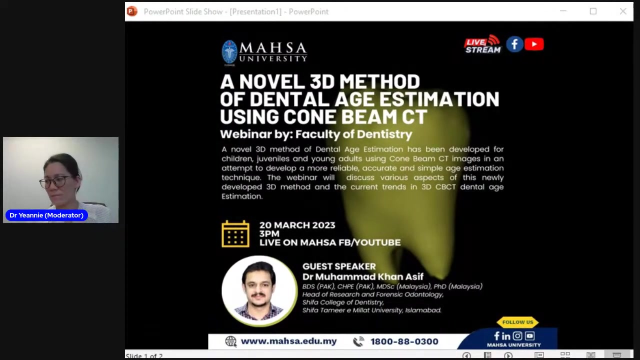 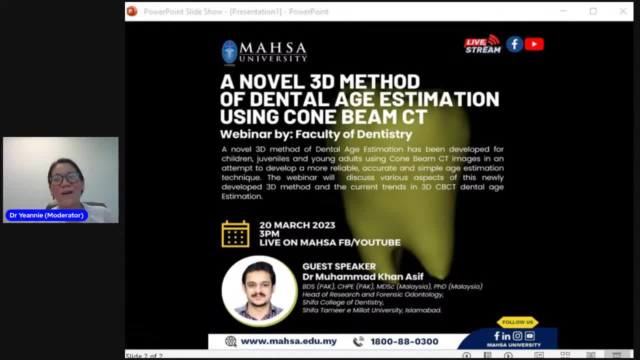 We are excited to have you all here today as we delve into one of the most important aspects of forensic dentistry, So dental age estimation. Dental age estimation plays a crucial role in many areas of our profession, from identifying the human remains to determining the age of suspects in criminal investigations. 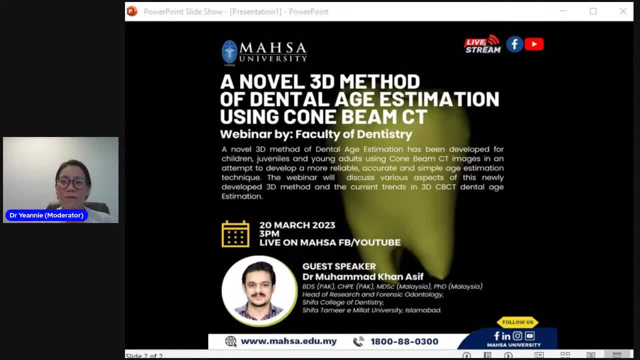 So, with the advent of CBCT technology, we now have a powerful tool at our disposal for accurate and reliable dental age estimation. Today, we have an esteemed expert, Dr Muhammad Khan Asif, who will be sharing his insights and experiences on this topic. 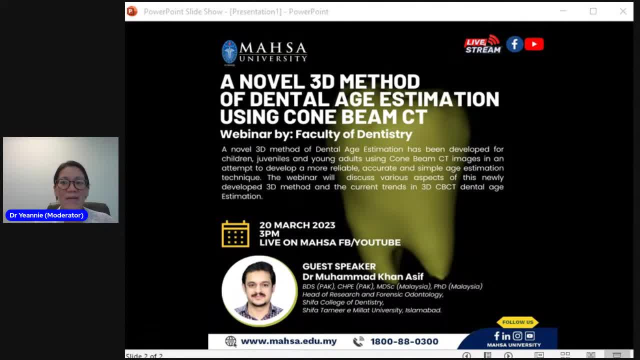 So a brief profile of Dr Muhammad. He's a forensic odontologist specialized in fetal, child and adult dental identification and age estimation. He and his core researchers have introduced a new method of computer-assisted animated superimposition in bite mark analysis for identification of the victims and criminals. 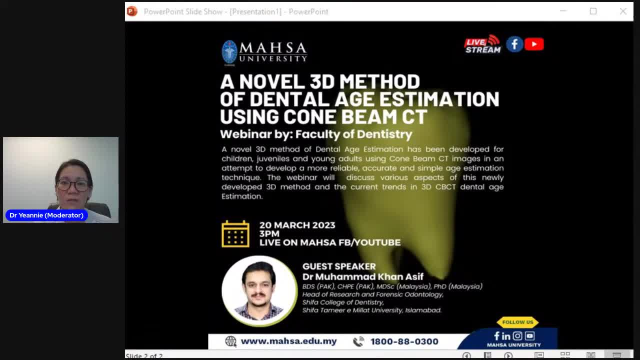 Moreover, these specific methods of dental age estimation have been developed by employing artificial neural networks Classified as ANN. He has also researched and published on prints conferral based on bone microstructural measurements using CBCD. He and his core researchers are the first one in Southeast Asia. 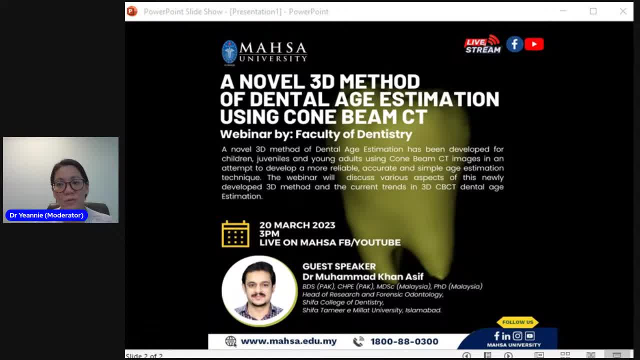 who have introduced the method of dental age estimation: volumetric analysis of dental structures using CBCT images for age estimations in adults. He specializes in CBCT image analysis and other 3D modeling software like Mimix, Freematics and Simplant. So Dr Muhammad has published 23 high-impact research articles. 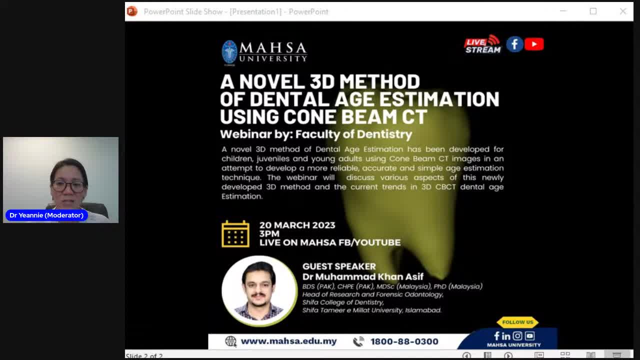 in the WOS or Web of Science index journals in the last six years and still counting. and he's definitely one of the few forensic odontologists in Pakistan and he's the first forensic odontologist with a PhD degree in oral and nasophacial forensic imaging in South Asia. 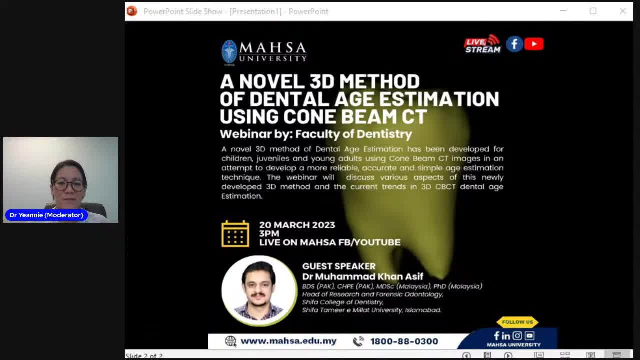 So, my dear audiences, please sit back, relax and explore the fascinating world of dental age estimation via CBCT. If you have any questions, you may actually post in the comment box below And I will direct it to Dr Muhammad, which is now already on the screen with us at the end of his talk. 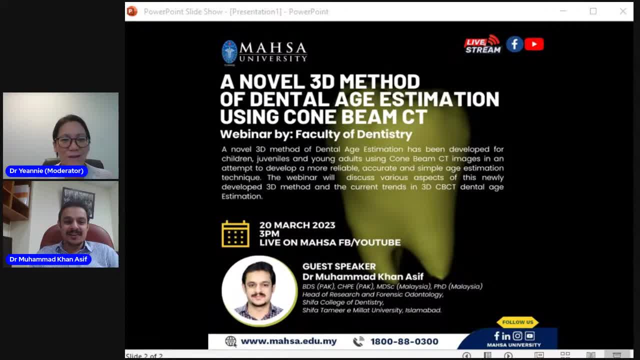 All right. so, hi, Dr Muhammad, a very good afternoon to you. Yes, so now I will pass the floor to you. Yeah, thank you. Okay, Thank you, doctor, I'll share my screen. Yeah, you can share the screen. 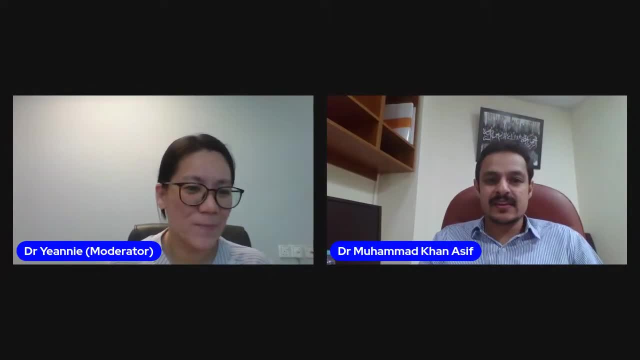 Let's see, Okay. Okay, I'll remove mine first. So now we should wait for Dr Muhammad to share his screen, then he can proceed with his talk. Yes, just give me a second. Yeah, sure, sure, Okay. so can you see my screen? 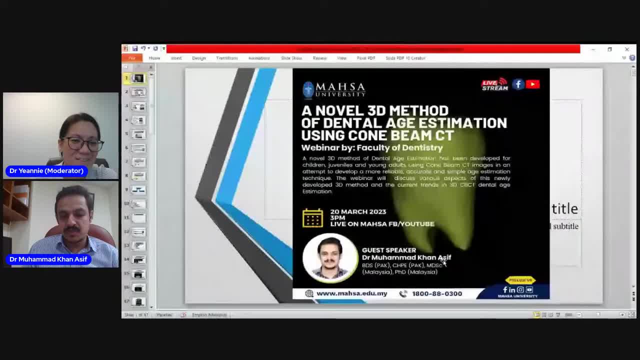 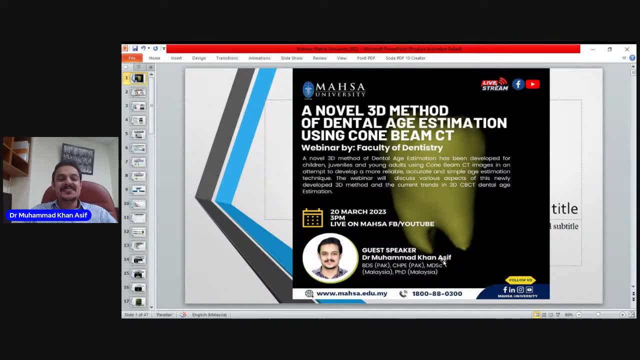 Yeah, Shared screen. Yes, doctor, Yes, yes, I can. Okay, so now I should pass the floor to you. Thank you, doctor. Okay, okay, So good afternoon everyone, And assalamu alaikum. 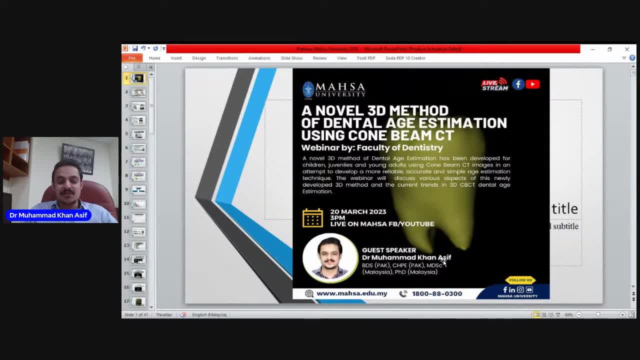 I hope all of you must be enjoying good health. Thank you very much, Dr Yanni, for your kind comments and welcoming remarks. I would also like to thank Professor Dr Prabhakaran Nambia and Massey University for inviting me to take part in this talk. 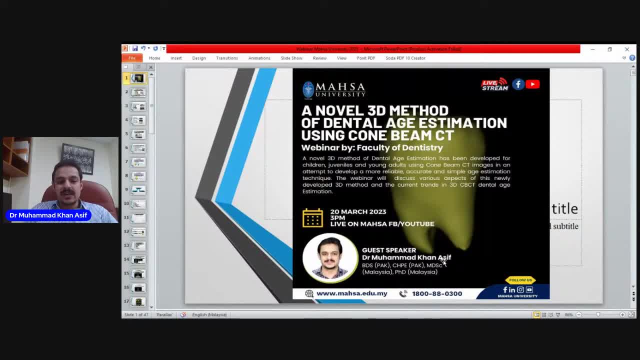 Thank you very much, Dr Yanni, for your kind comments and welcoming remarks. I hope all of you must have a pleasant day as well. I'm very proud to welcome Dr Dr Yanni in the June 9th round. 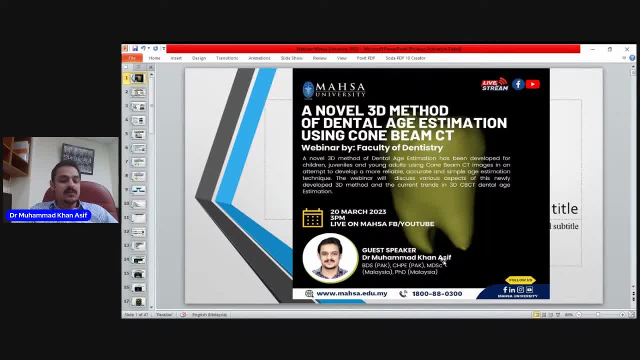 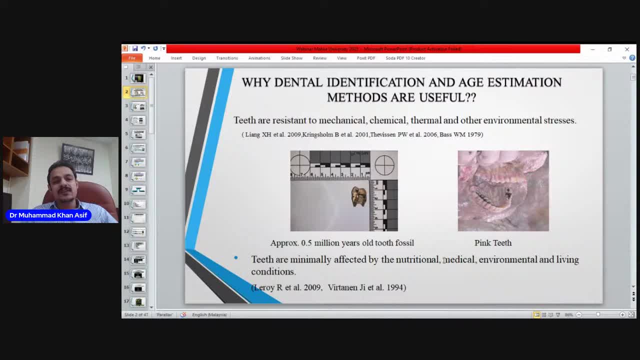 Nowサ. Thank you so much for this meeting My pleasure. Every individual is a fascinating body And I'm so pleased to see you on this virtual event. Thank you, Bye. and they can withstand physical, chemical, mechanical and nutritional stresses to a great extent. 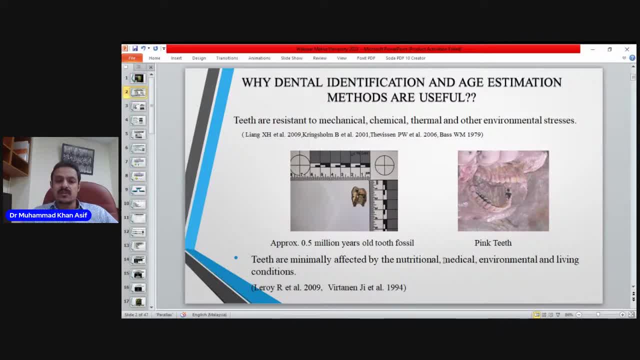 And that's why they can be used quite effectively for the identification and age estimation. And recently we have been working with the geology department at the University of Malaya And the picture that you see on the left side is actually a tooth fossil. 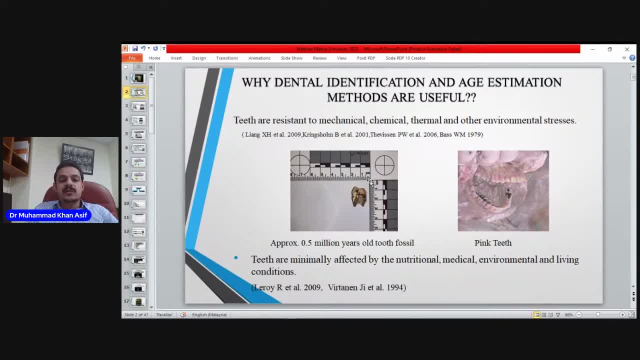 which have been shared with us by the geology department, which dates back to about 0.5 million years old. So you can imagine how the teeth can withstand all these harsh environmental conditions, And that's why they can be used very effectively for identification and age estimation. 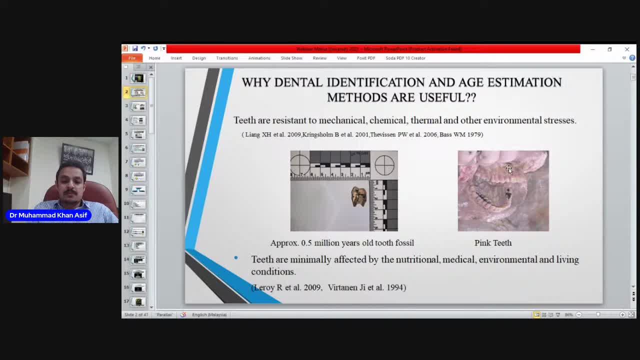 And, similarly, people say that dead people cannot talk, but we, as forensic odontologists, believe that they can talk to us And the picture that you see here is the pink teeth, which is indicating the accumulation of hemoglobin in the dentinal tubules. 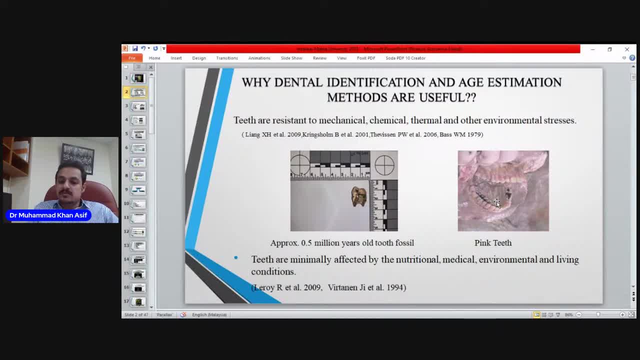 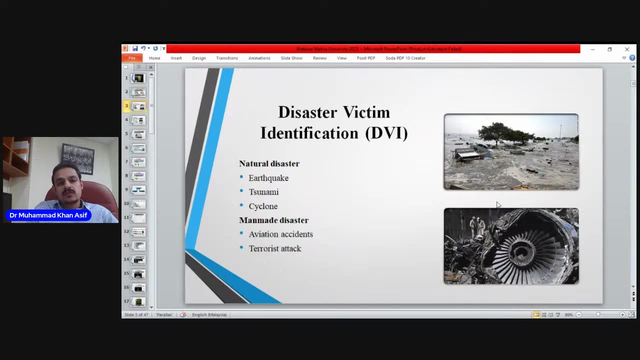 And this mainly occurs after the torturous death, So they can talk to you as well. So that's why teeth plays a very significant role in the identification and age estimation. Now, when we talk about the implementation of the legal justice system, of course dental needs or dental age estimation plays a very important role. 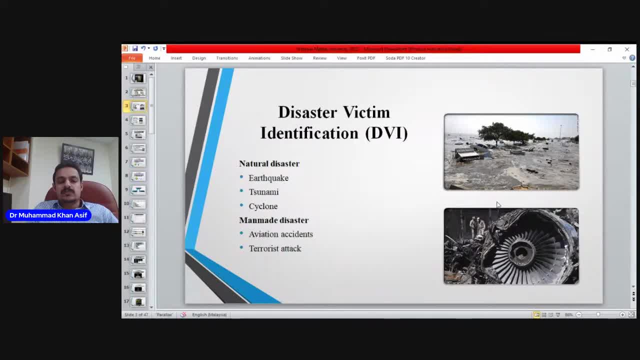 In the civil and legal justice and criminal investigations to implement the legal justice system. But besides that, it plays a very significant role in disaster victim management. And when we talk about disasters, whether they are natural or manmade, in the form of, in the form of earthquakes, tsunamis, aviation disasters, 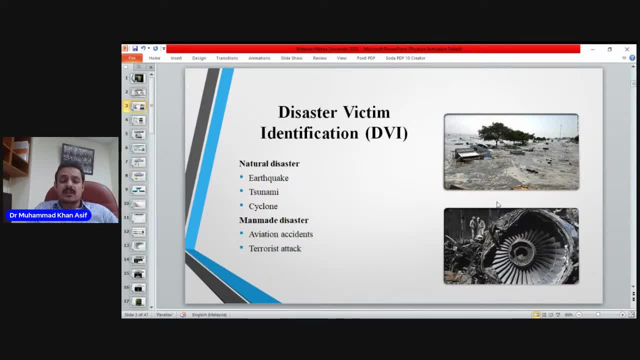 they may be sudden, unexpected and they involve large amount of loss of life, And it's very difficult For the local government resources to manage such a situation on such a large scale, especially when we talk about the developing world. So forensic odontology can play a very significant role, especially dental age estimation, one of the aspects of it. 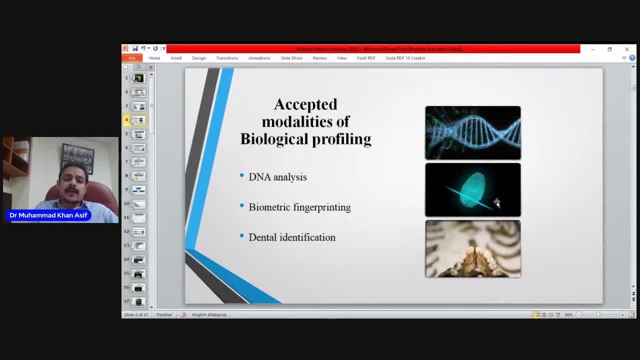 And why is it important? Because, according to the Interpol, there are three primary identifiers that can be used for the identification purposes: DNA analysis, biometric fingerprint printing and dental identification. And dental identification is one of the simple and quickest method of identification. 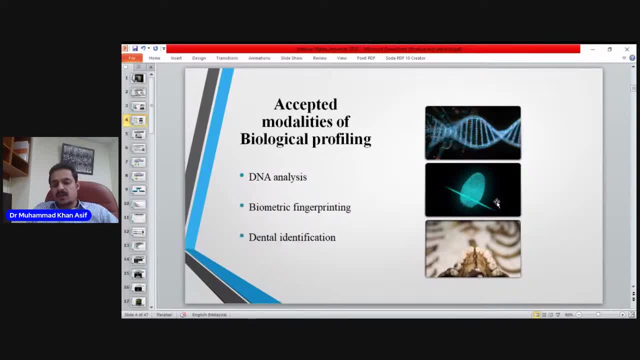 As far as these three primary modalities are concerned, I'm not going to the detail of the limitations and the merits of each of these modalities, But dental identification is one of the means and, especially when, even if it's DNA analysis, dental DNA is one of the reliable sources as well. 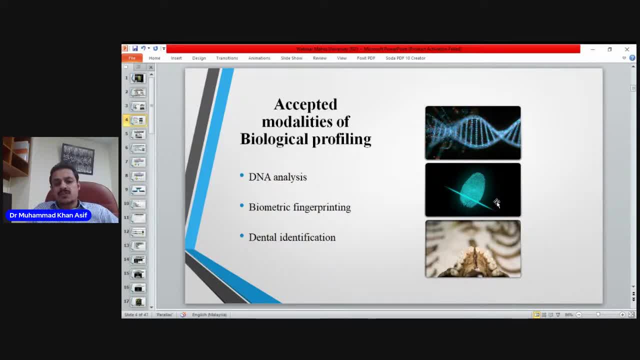 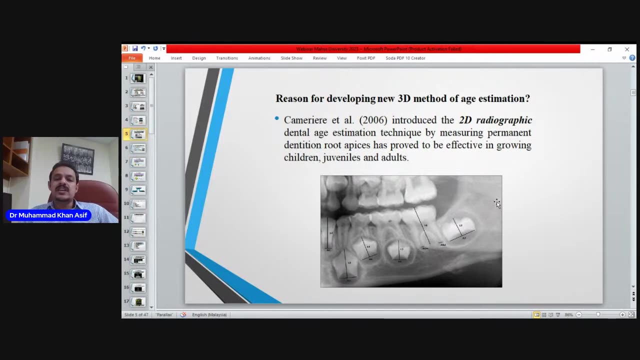 Why? Because, as I said, teeth can withstand harsh environmental stresses to a greater extent. That's why they can also be a source of DNA for the identification purposes. Now, coming back to the dental age estimation and why we felt the need of developing this new method of dental age estimation, based on the CBCD image analysis. 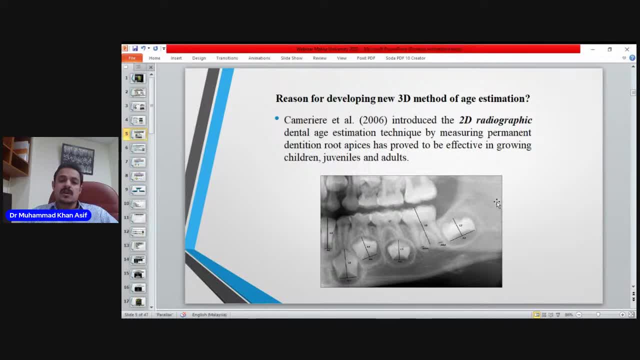 Now chemo here And they core researchers. they've introduced a new method in 2006 of estimating dental age by assessing the open apices of the left sound mandibular teeth And this method proved to be very effective and was validated all over the world on various populations. 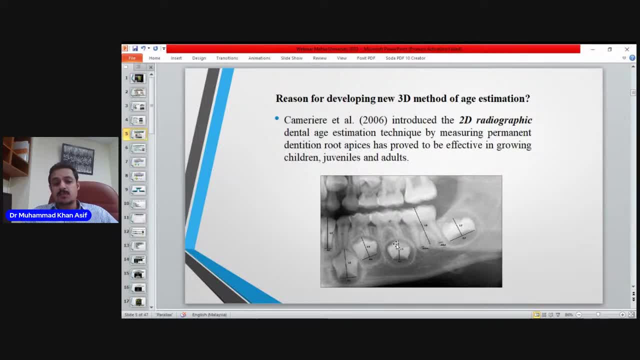 But we all know that, despite effectiveness, this is the beauty of research, that you keep on exploring more reliable methods, more accurate methods. And we all know that they developed this method based on the panoramic radiographs, which is a two-dimensional radiographic modality. so, uh, because two-dimensional radiographs have some limitations and 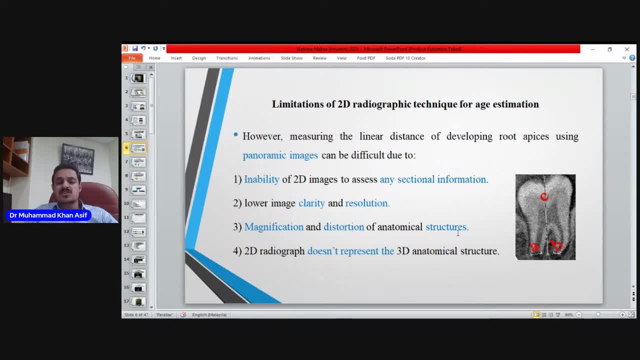 some of the major limitations is that you cannot see any sectional details, uh, using two-dimensional radiographs, because it gives you only the two-dimensional view, and especially when it comes to magnification, distortion or resolution, the two-dimensional radiographs have limitations because of various reasons. uh, those of you who are aware about the 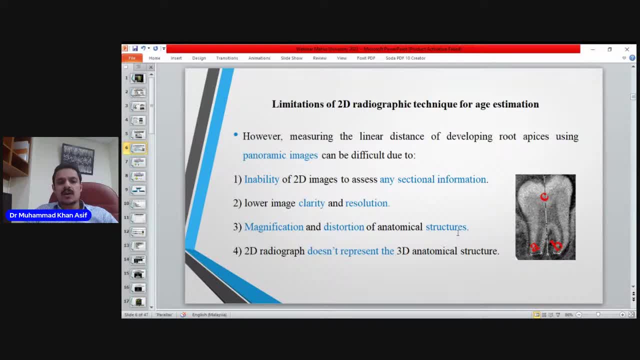 radiographic images and how they're taken. uh, you can see that in two-dimensional radiographs the magnification occurs because of phase reasons. let's let's talk about the panoramic radiographs. in panoramic radiograph, the distance between the film and the anatomical structures which you want. 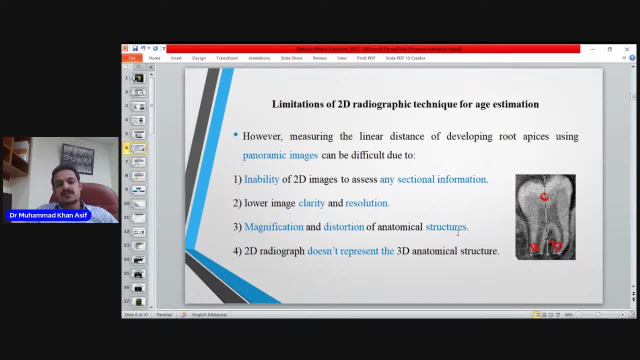 to image in the radiograph. they're at a distance from each other and that's because of that distance, uh, there's a magnification. and similarly, if we talk about the x-ray source, inclination or orientation, it's also at five to eight degrees upwards. so because of that, there's also 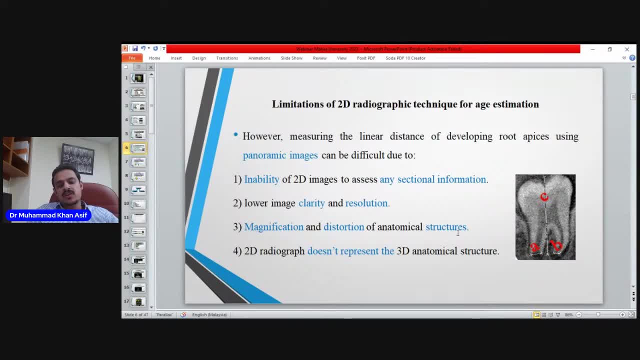 magnification. so these are some of the factors, uh, which- uh, that's what we thought- that we can develop a more reliable method based on the three-dimensional radiographic imaging modality rather than using two-dimensional radiographs. now, another thing which is uh logical as well: 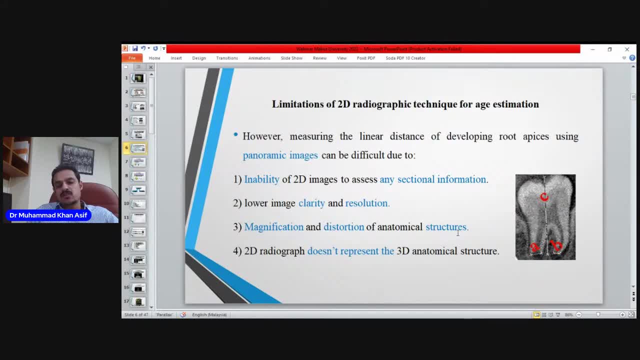 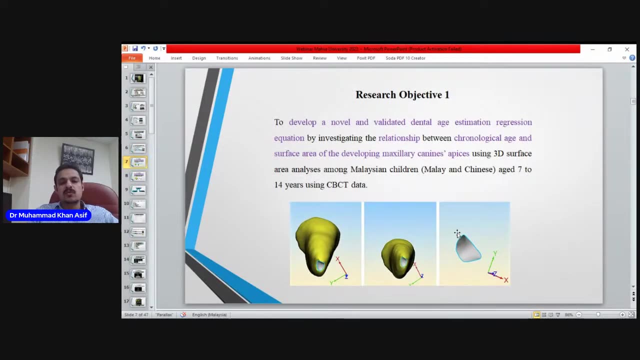 that it's. it's more logical to assess the three-dimensional anatomical structure, which in this case is street uh, by using the three-dimensional imaging modality rather than using the two-dimensional anatomical radiographs. so, uh, the first research objective of our study was to develop a age estimation equation- regression equation, by investigating the relationship between 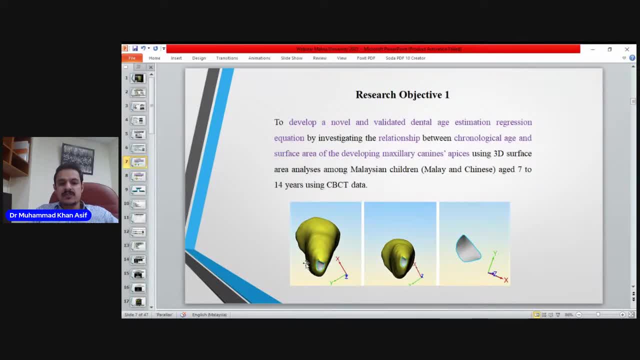 chronological age and the surface area of the developing maxillary canine emphasis using cbct of auxiliary canines aged 7 to 14 years of age. so this was our first objective and we wanted to see a correlation between age and the developing surface area of the canine emphasis. 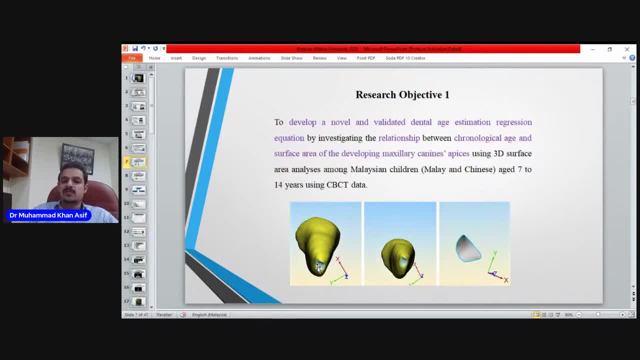 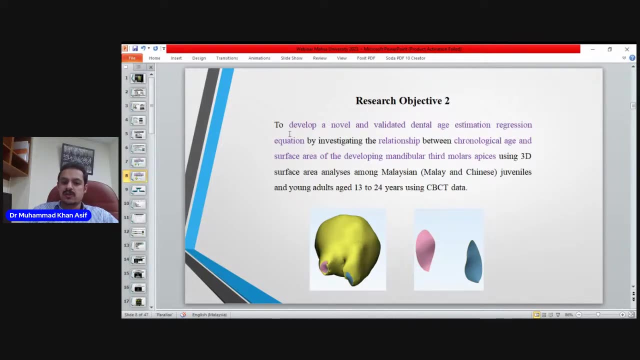 among 7 to 14 years of age. so the first objective was addressing the to develop the age estimation equation for children of aged 7 to 14 years. the second objective of the study was to develop again another age estimation regression equation by investigating the relationship between the chronological age and surface area of the. 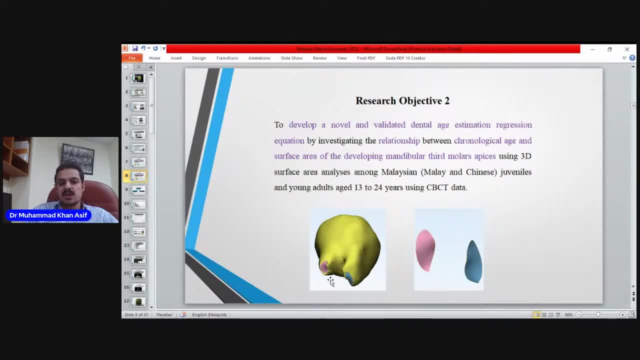 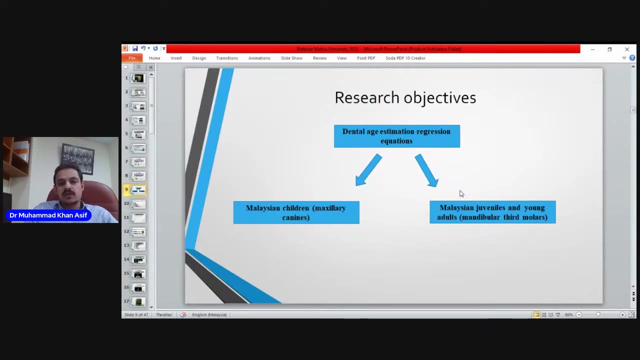 developing mandibular third motors appuses and among juveniles and young adults aged 13 to 14 years, using cbct data. so these were basically the two research objectives: one was to develop an equation or regression model, uh for children uh based on canine root apices development using CBCT images, and the second one was to develop a regression equation. 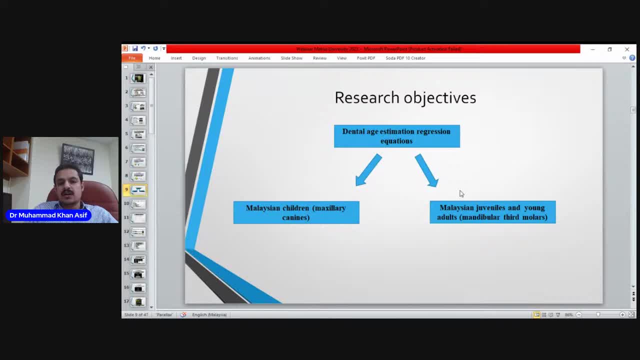 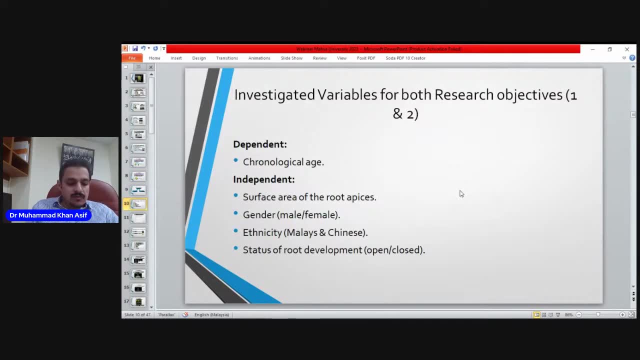 for Malaysian juveniles and young adults age 13 to 24 years of age using CBCT images. Now, the variables that we used, that we investigated for the research objective for both of them were the chronological age, because actually we wanted to correlate whether there's any relationship. 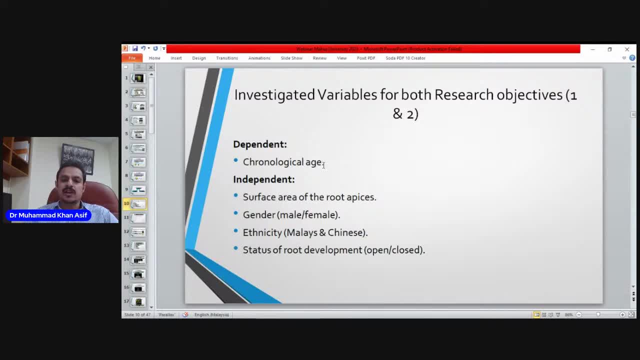 of the changes in the surface area of the developing root apices with age or not. So we took it as a dependent variable or output variable and the independent variables on which we wanted to test whether the chronological age depends on these predictive variables or not. 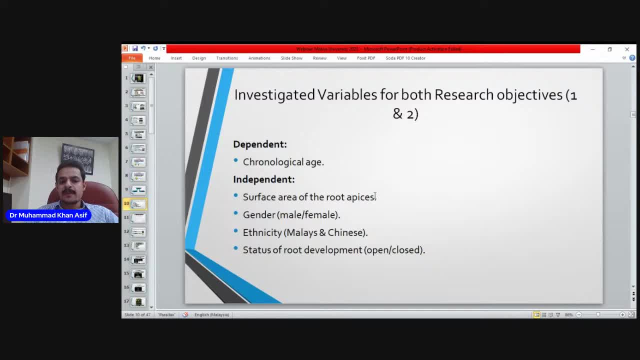 So we have the surface area of the root apices. in the case of first objective, it was for the canines. in cases of the second of the objectives, it was for the third molars. Then we wanted to see the gender effect, whether the gender is fitting with the model or not. 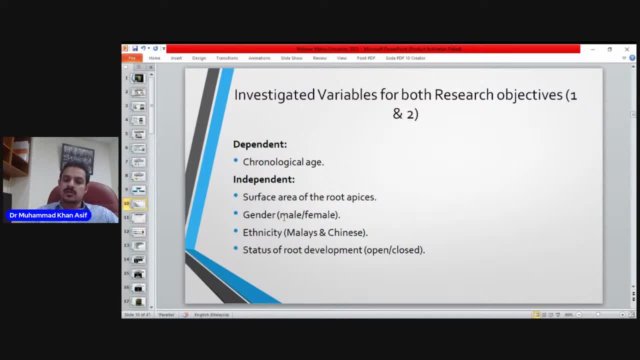 whether there's any effect of gender on the root development or not. Similarly, ethnicity, because Malaysian Chinese, although they both belong to the mongoloid race, but some of the studies have shown morphometric variations in both of these ethnic groups as well. So we wanted to investigate the effect of ethnicity on the age estimation as well, and also on the age. 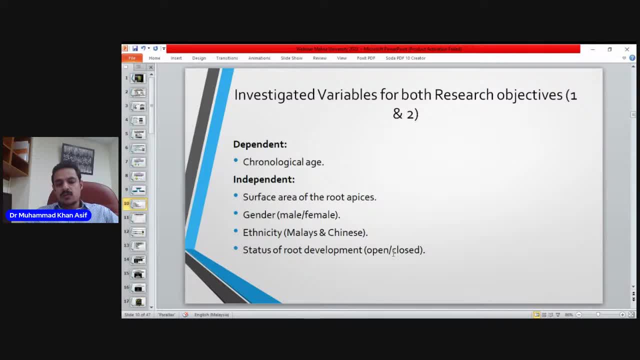 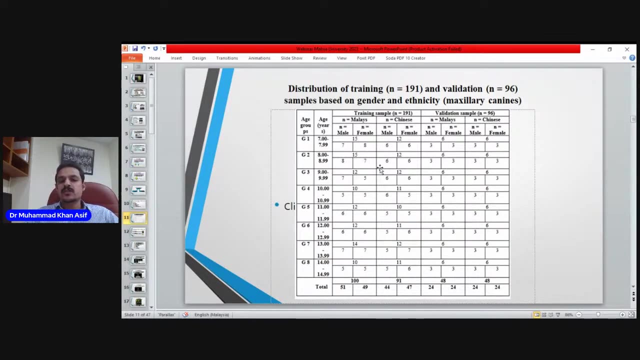 estimation, regression equation And the status of the root development, whether the root is open or closed. So we wanted to see the effect of the status of the development on the age estimation model as well. Now for the first research objective which I mentioned, that we developed it for the children age 7 to 14. 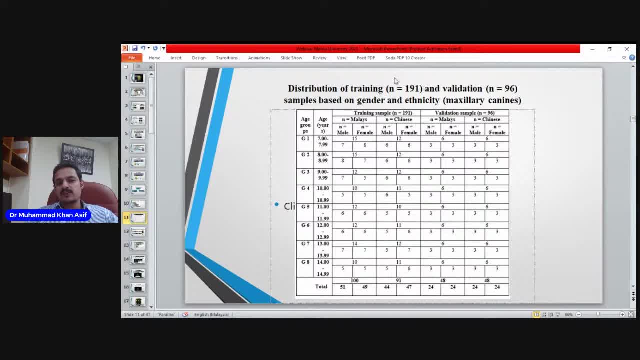 years and we used canines. We used 191 training samples on which we developed the model and then, after developing the model or tested it on 96 validation sample on which we validated our regression equation which we have developed. So we have further divided them into eight age group, from seven years to 14 years of. 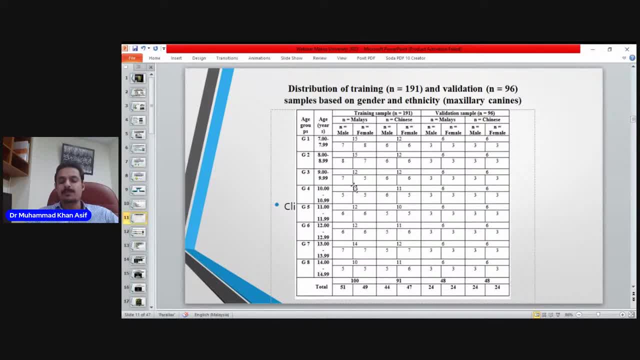 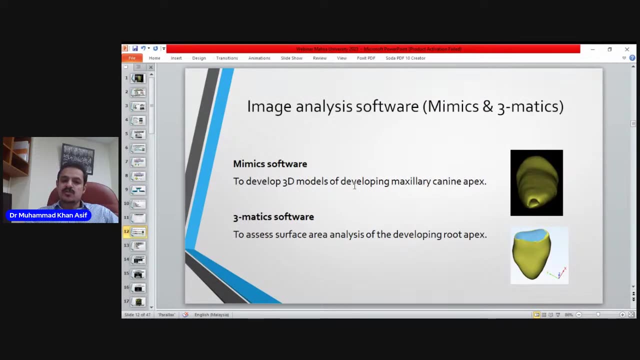 age for equal distribution or stratification of our sample, because if the sample is not stratified accurately, it will give you bias results when you develop a regression equation or when you want to see a strength of correlation. Now, as the main idea was to develop the 3D models, 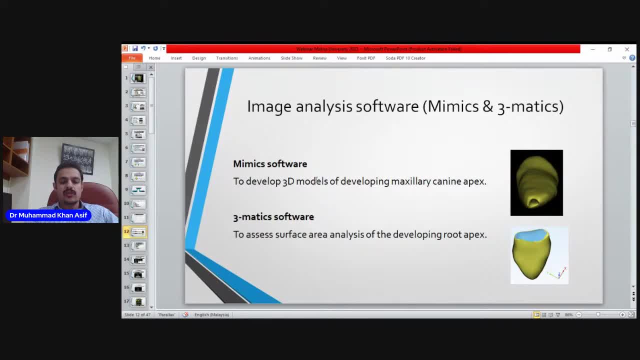 of the developing teeth. so we used MIMIC software and 3MATIC software for this purpose. MIMIC software was used to develop the 3D models of developing maxillary canine apex, as you can see over here, and 3MATIC software was used to assess the surface area of the developing root apex. So 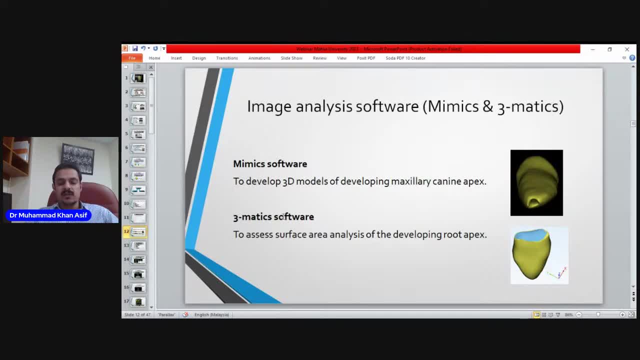 the surface area of the root apex is the surface area of the root apex. So the surface area of the root apex area was measured using the thematic software. So once we developed the 3D models in MIMIC software we transported them to thematic software for surface area analysis. 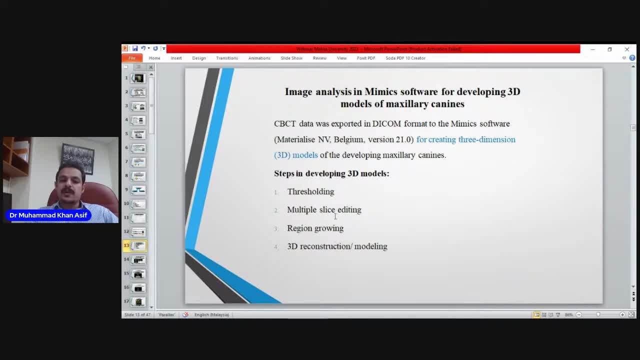 There were different steps that were involved in developing the 3D models in MIMIC software to create the 3D dimension models of the maxillary canines. because we used maxillary canines for the first research objectives, The first step was to thresholding, then multiple slice editing. 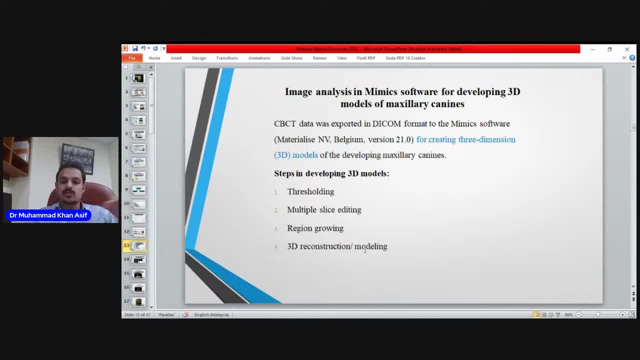 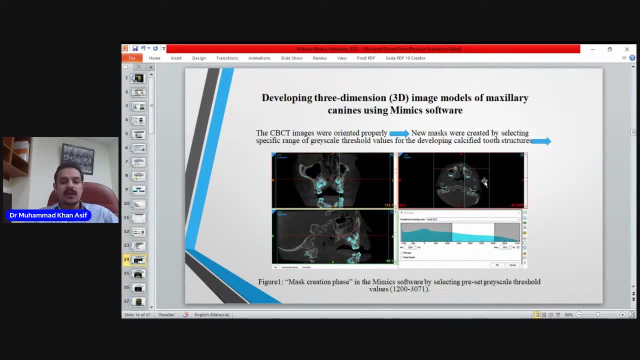 region growing phase and 3D reconstruction or modeling. Let's go through them step by step. First was the thresholding. Now those of you aware about the radiography or radiology, at this stage we assign the grayscale threshold value to each of the voxels, based on the density. 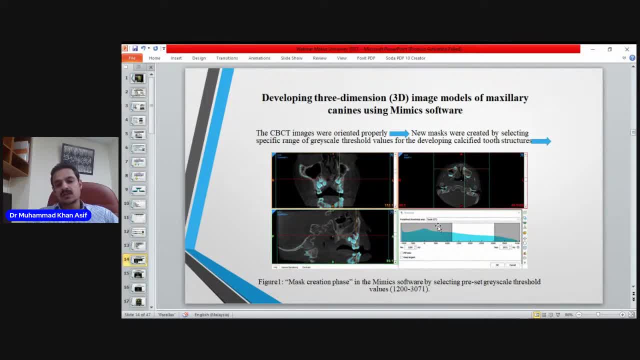 of those structures. Now, as I mentioned at the start of the presentation, the teeth are the most calcified structures of the human body, So the density is very high and, as a result, because of this high calcification mineralization, you can clearly demarcate the 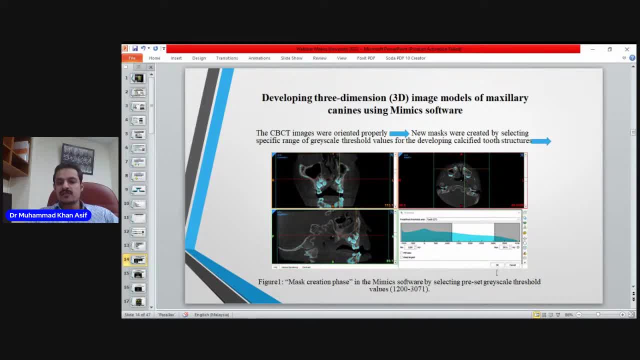 grain dental structures from the surrounding structures. So we have assigned a grayscale threshold value as you can see here, preset grayscale threshold value of 1200 to 3071.. But we have to keep in mind one thing: that these are the developing teeth, So mineralization is taking. 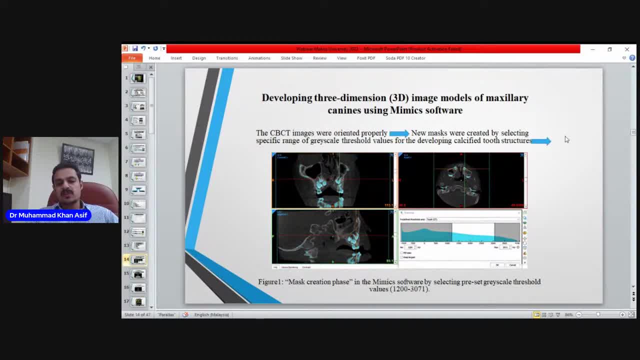 place, calcification is taking place. So in some of the cases, we saw that even the software was not accurately identifying the growing maxillary canines or mandibular third molars on which we were developing our model on And, as a result, what we did, we wanted to cross check whether 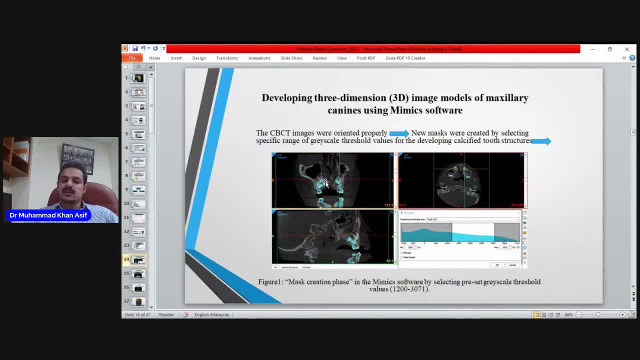 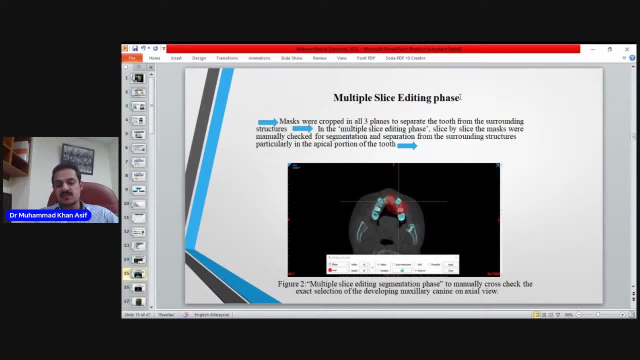 the software has accurately selected the growing teeth- Maxillary canine or not. So we used another tool, which is multiple slice editing phase And, as the name suggests, we were able to add or remove the masks which the software has not accurately selected. So this tool helped us to cross check whether the 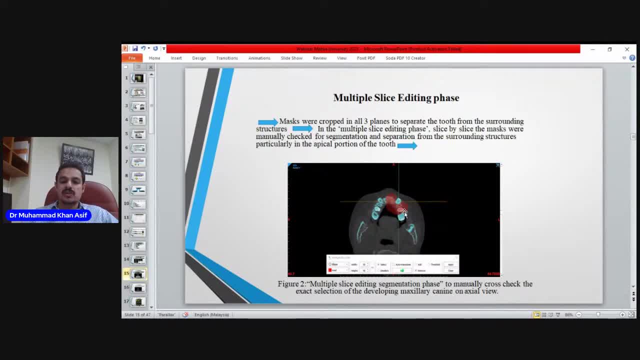 software has accurately selected the calcified tooth structure or not. Now why this phase was important. See, we use the voxel size of 0.30 millimeters and the voxel size has an effect, which we call it the partial volume averaging effect. And if you use the smaller voxel size, the resolution can be enhanced. 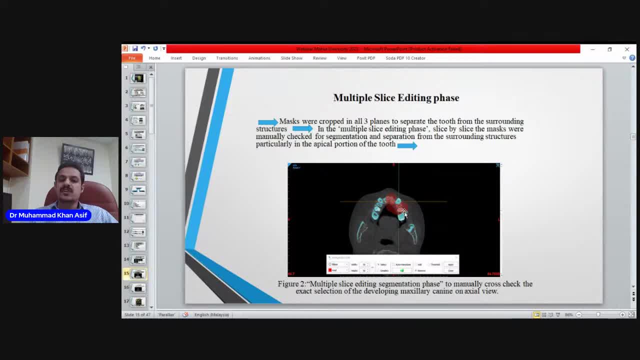 But because of some of the limitations, the scans that we have included in our study had the voxel size of 0.30 millimeters And, as a result of partial volume averaging effect, sometimes the software was not accurately demarcating the small, minor structural details or was not selecting the 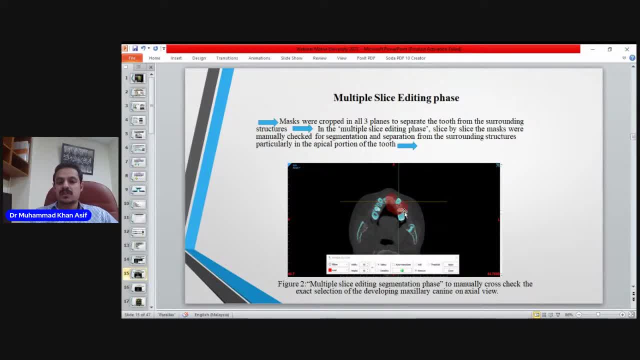 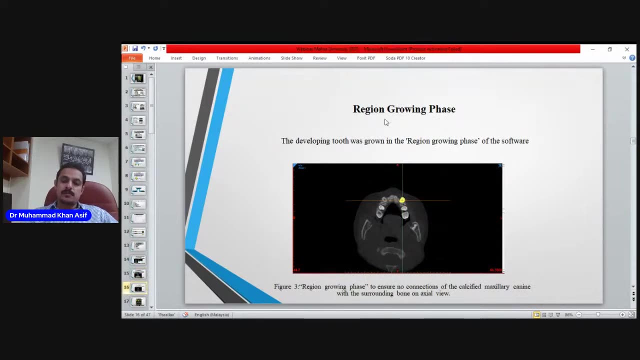 proper calcified structure of the developing maxillary canine, as well as for the mandibular third molars. so that's why this tool was very helpful, because we made sure that we are selecting the tooth, the brain teeth, very accurately and region growing phase. now. this phase is important. 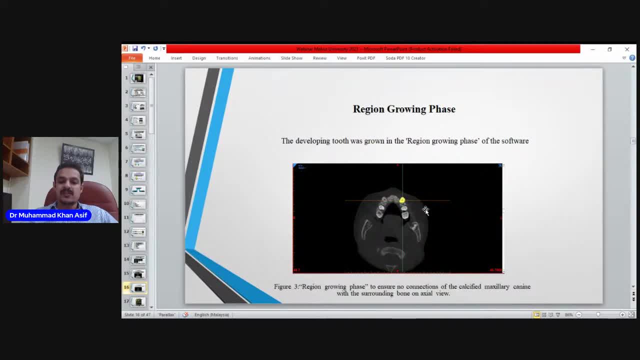 because you just want to see the growing maxillary calcified structure of the growing maxillary canines. you don't want any other structures or other teeth. so in this we have separated the teeth with which we were concerned and we have removed all the other areas we have. 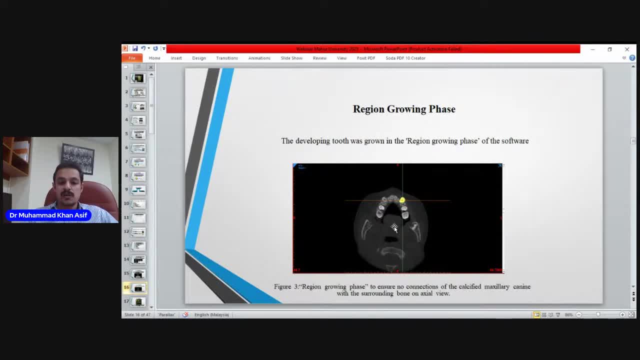 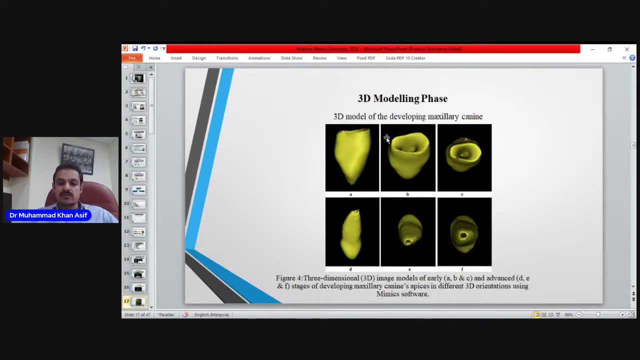 grown the region which we wanted to develop as a 3d model, and this is how the 3d models were developed and you can see why. this is the early stage of development of the maxillary canines, and so this is what we are looking for in this three-dimensional radiographic model. this is 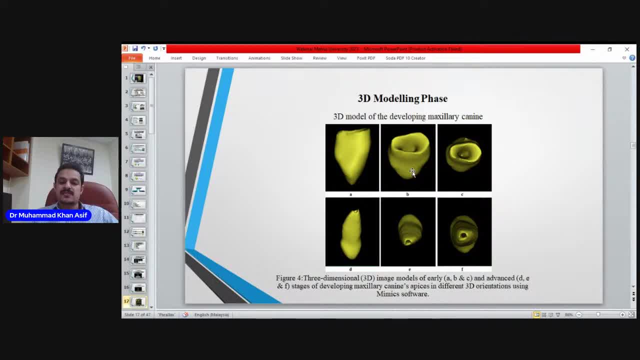 a very advanced stage and if you compare this with the two-dimensional radiographic methods in which we assess the age or estimate the age based on the root abscess, it's very clear you can see the margins of the developing maxillary canine very accurately in comparison to the two-dimensional 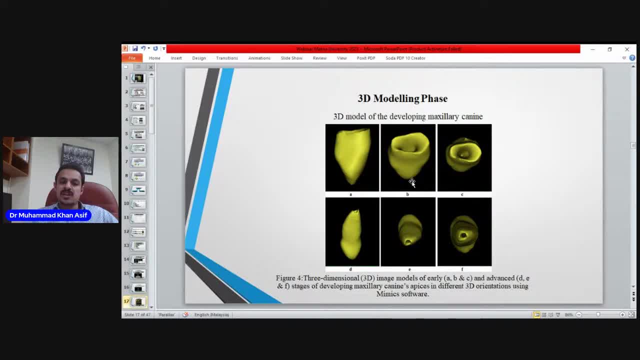 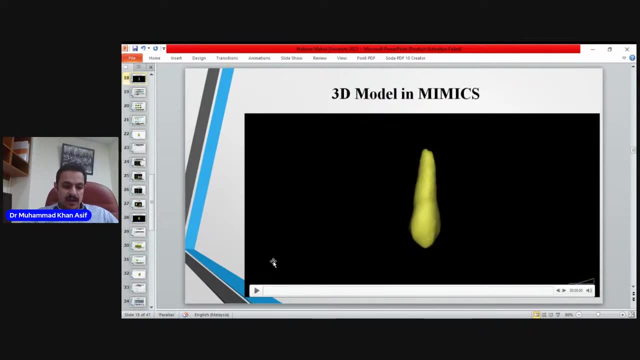 methods, and this is the reason that why we wanted to develop this method structure using three dimensional imaging tool, rather than assessing the same three dimensional anatomical structure using two-dimensional radiographs, which, mainly panoramic radiographs, were used. now, this is how I have this video, that this is. 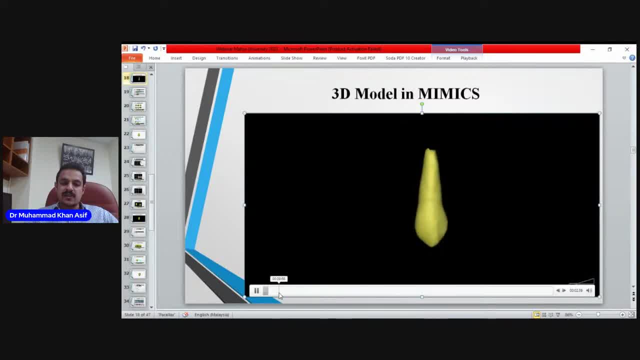 how the three-dimensional models of the maxillary canines are seen on mimic software once the 3d models are developed. so this is slightly advanced stage of the maxillary canines. this is the apex you can see. even you can see the bulb canal and the chamber. 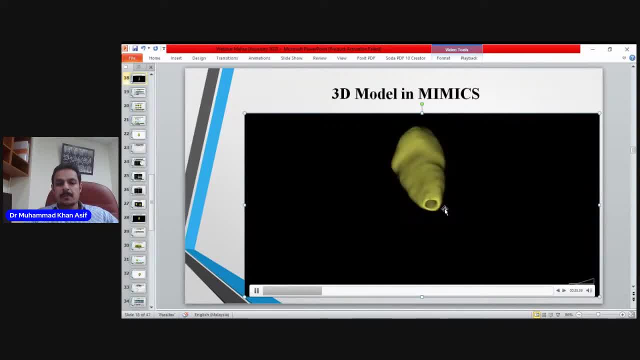 inside as well, and the best thing is that you can move it around because you want to assess the developing root apex very accurately. so this is how you can zoom in, you can zoom out, you can see all the structures: the labium, the palatal, the mesial and the distal root surfaces. 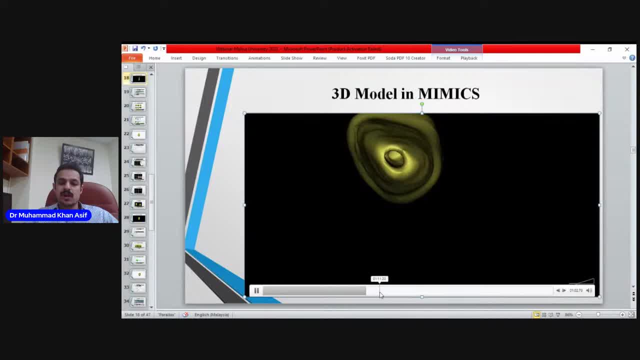 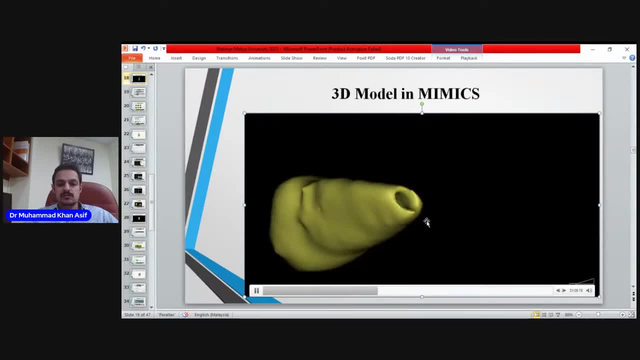 like you can see over here. you can zoom it in, zoom it out. the margins are very clearly defined in this three-dimensional image model of the maxillary canine. okay, now this is another canine. you can see one thing which observed was a bit strange as well: in some of the cases the root development was not uniform. in 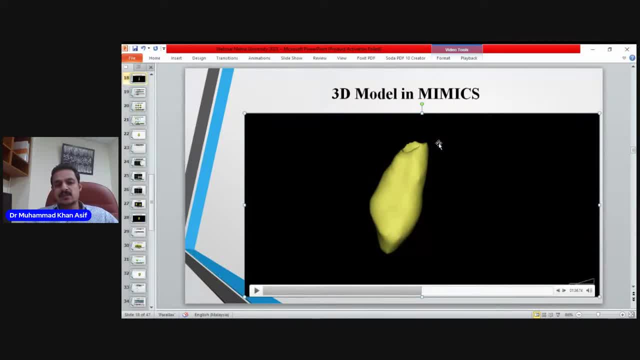 all the three planes. for example, in the labial, palatal, mesial distal, like in this case, you can see that the palatal root is less form as compared to the labial aspect. so this was the Advantage, because you were looking at the three-dimensional structure. so we have also recorded these values as 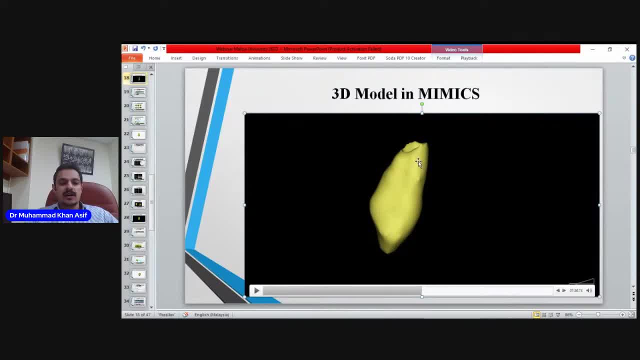 well, and maybe future studies can also look at that which of the surfaces of the root apexes develops first as compared to the other surfaces. so this was an advantage, because we are looking at the three-dimensional models rather than two-dimensional images and you cannot assess this using the panoramic radiographs or two.